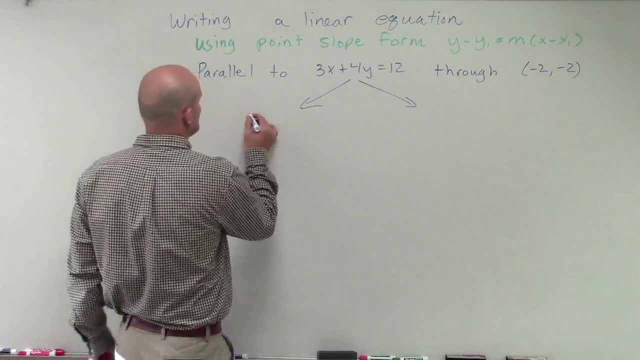 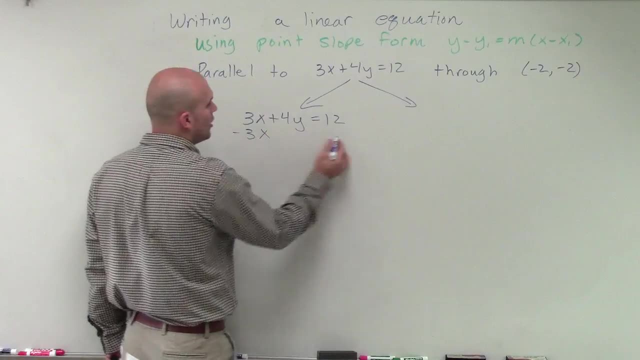 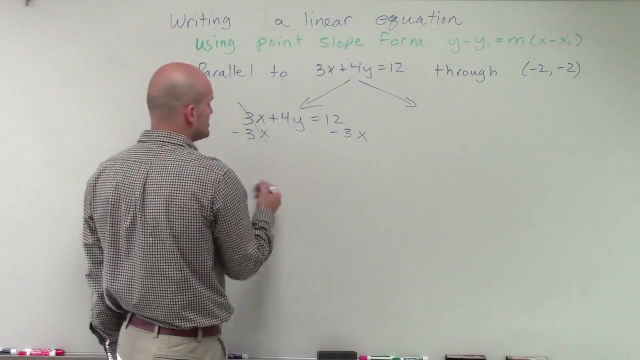 just converting everything this over to slope intercept form. So I have 3x plus 4y equals 12.. Well, to put this in slope intercept form, I need to solve for my y variable. So I'm going to subtract the 3x which those will add up to 0 on both sides. Therefore, 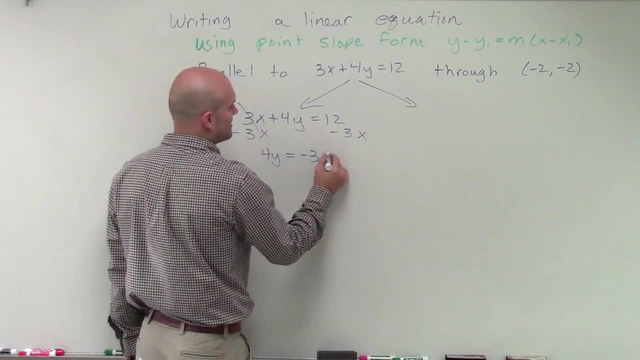 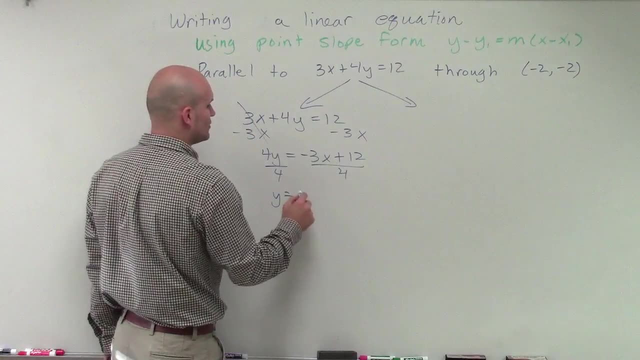 now I have 4y equals. I'm going to rewrite this as a negative 3x plus 12.. Then I divide by 4 on both sides and I get y equals a negative 3x plus 12 divided by 4.. But we 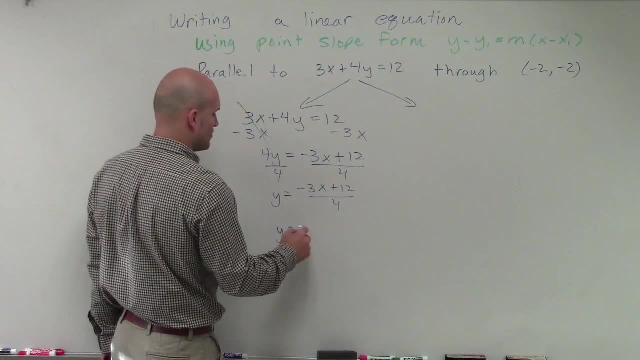 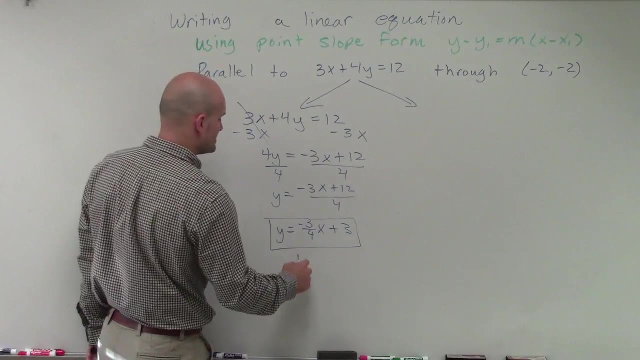 got to make sure we divide the 4 into both terms. to put in slope intercept form, So we have a negative 3 force: x plus 3.. So that is going to be our equation where we can see our slope equals a negative 3 force. Now there's another way you can do this without. 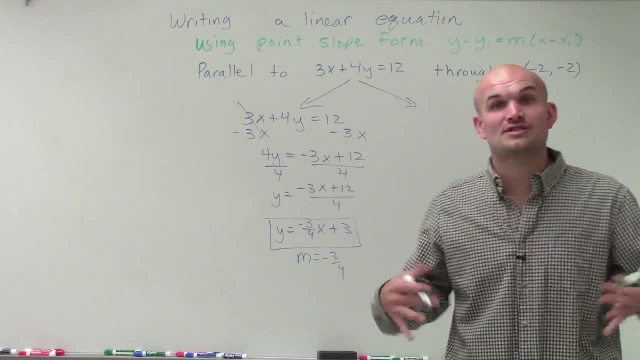 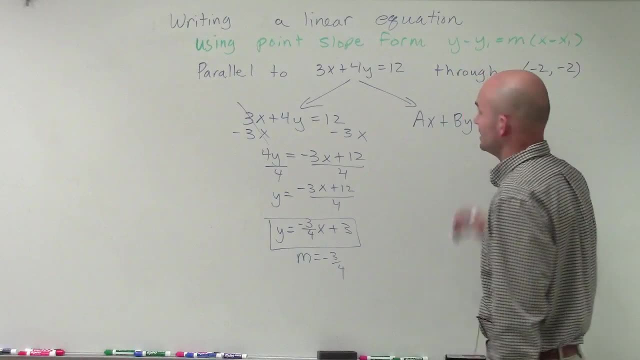 having to do all of that algebra but it really kind of takes a little bit more understanding of our standard form. So it will take a little bit more understanding of our standard form. So if we know standard form is ax plus by equals c And you have an equation that makes 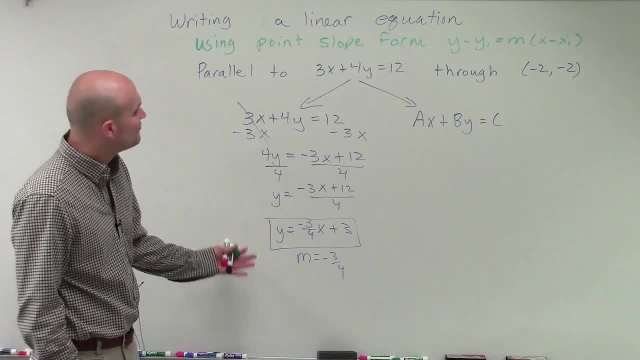 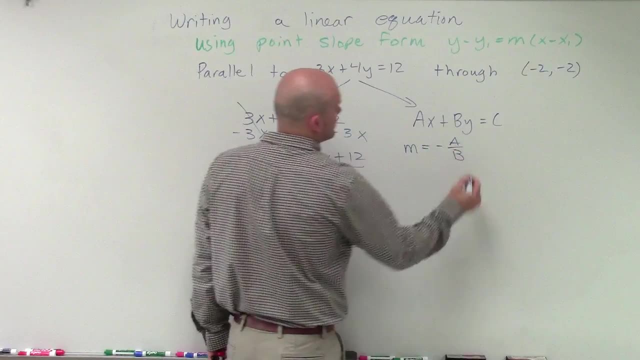 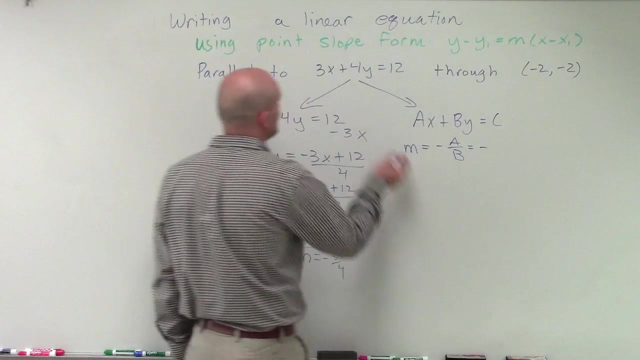 sure it's in that format To be able to find the slope, all we need to do is take the slope is equal to the opposite of a over b And that's pretty much it, And you can see that well. that equals opposite of a, which is 3,, over my b, which is 4.. So that's a very 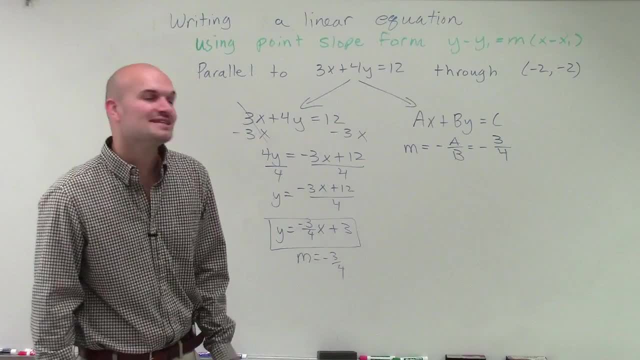 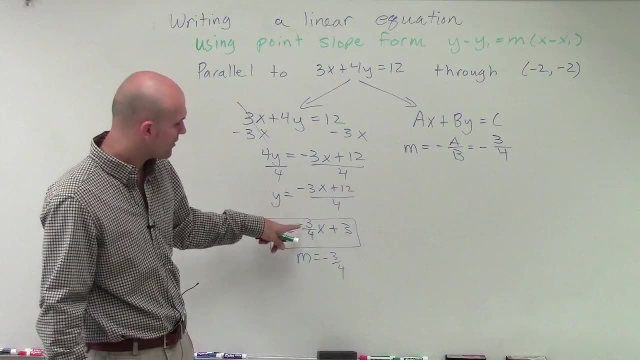 simpler, more simple way, I guess you could say, to find the slope, But a lot of times some students this just really hasn't too much understanding. You can see why this works is because when I solve for it I get that equation where I still determine the slope is a negative 3 force. However, 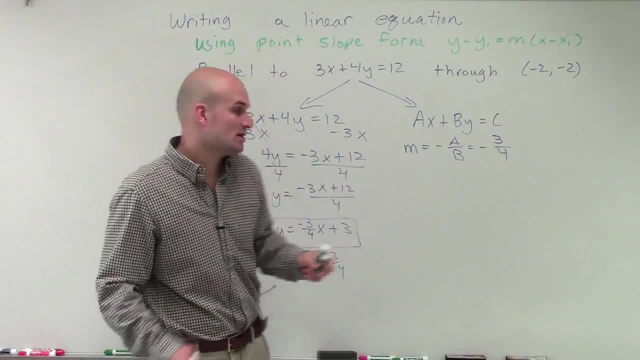 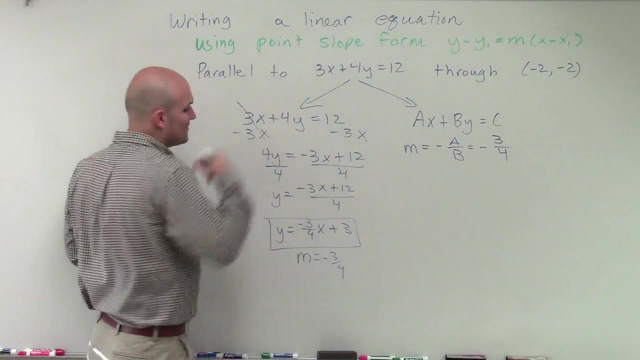 this is a little shortcut. As long as you understand this, this is a good shortcut to use, All right. So now we know what the slope is And if we're going to find a parallel line, we know that parallel line has to have the exact same slope. So therefore, I know that. 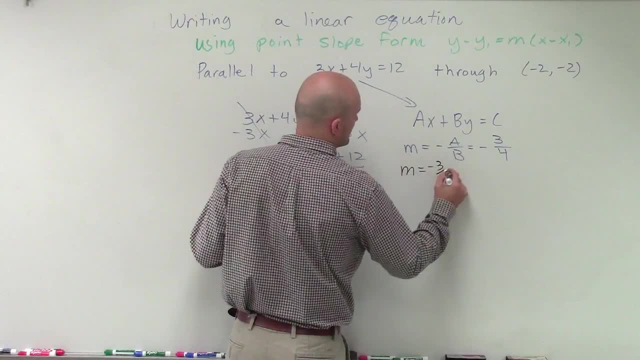 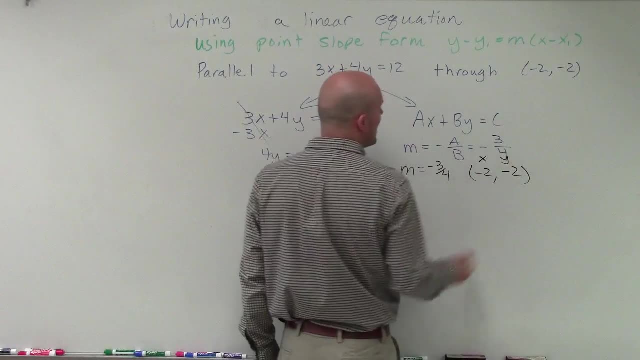 the slope is m equals negative 3 force And it has to be equal to the slope. So that's the slope And it has to go through the point negative 2 comma, negative 2.. Well, remember a point: we can label as an x and a y, But we don't want to label it as x and y. studying for. 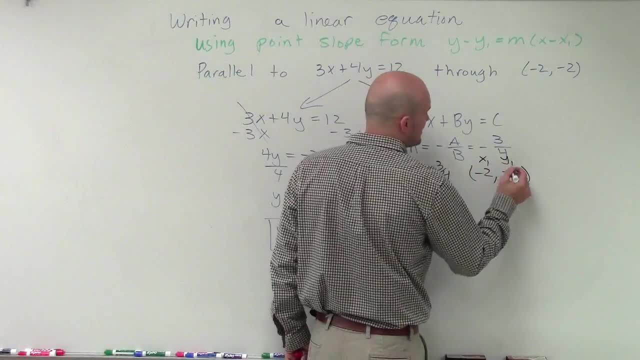 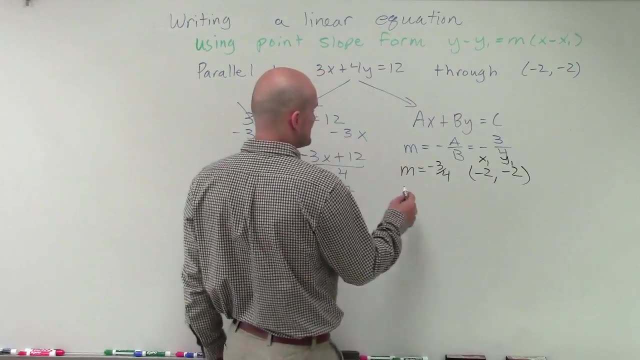 any point on the line. We want to label it as a specific point. So I'm going to label it as x1 and y1, which, looking at our point slope form, we can plug in for x1 and y1. So that's exactly what I'm going to do. I'm going to say y minus y minus negative y1,. 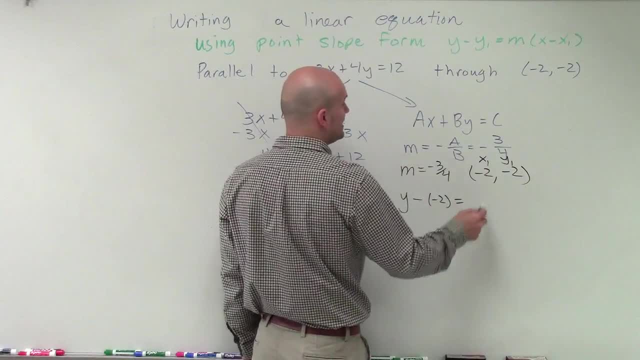 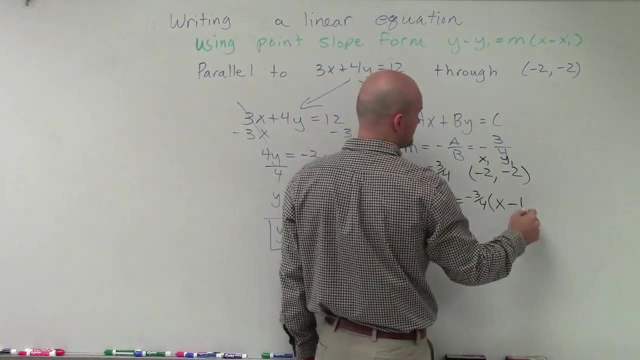 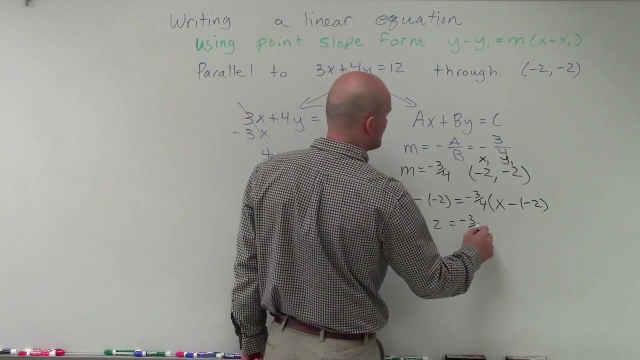 which is a negative 2.. So you got to make sure you apply your parentheses. Equals our slope, which is a negative 3, force times x minus x1,, which is negative 2.. All right, So now I simplified the left side, So that's going to be: y plus 2 equals a negative. 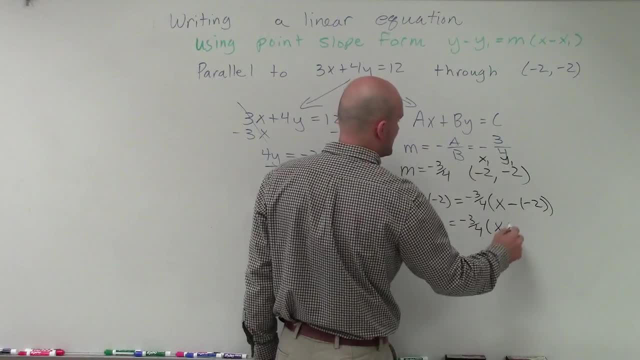 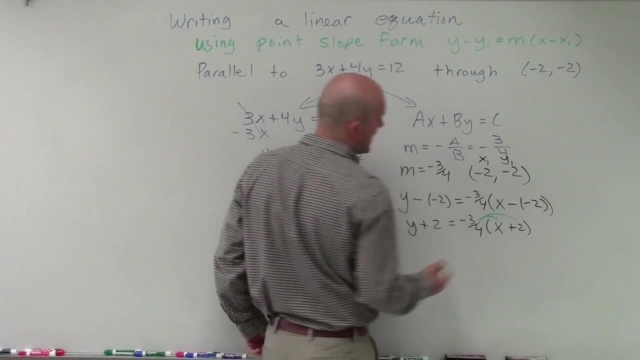 3 force. Let's simplify this parentheses, which will be x plus 2.. Now we can apply the discerative property, And I'll use a little coloration to make sure we multiply our negative 3 force times both of our terms. So therefore I have y plus. 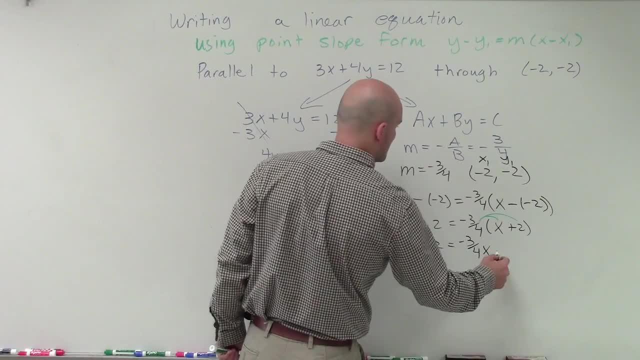 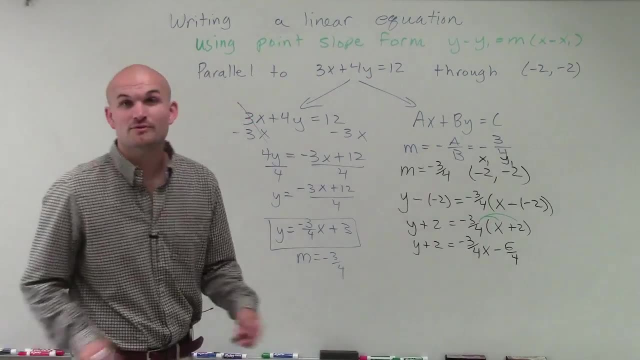 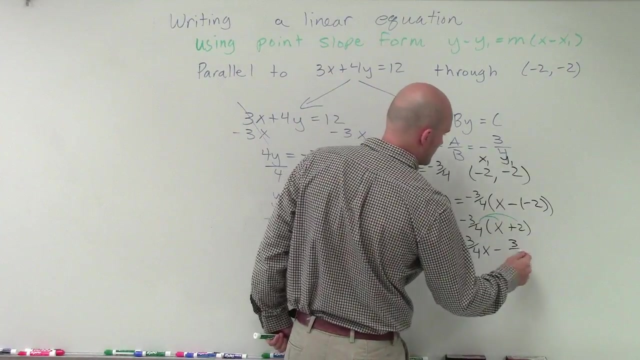 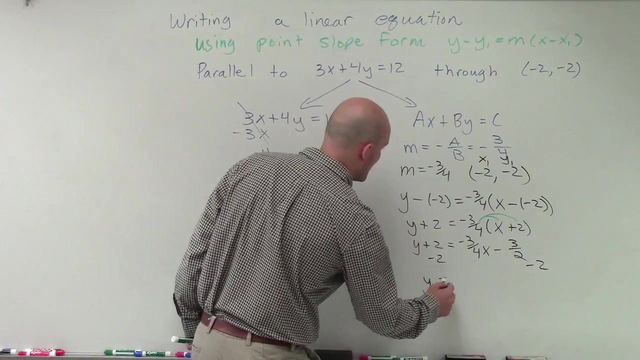 equals a negative 3 force, X minus 6 force. and that 6 force we know we can reduce down to 3 halves. so let's just go and reduce that now. all right, then I'll subtract 2 on both sides using my inverse operations. therefore I have Y. 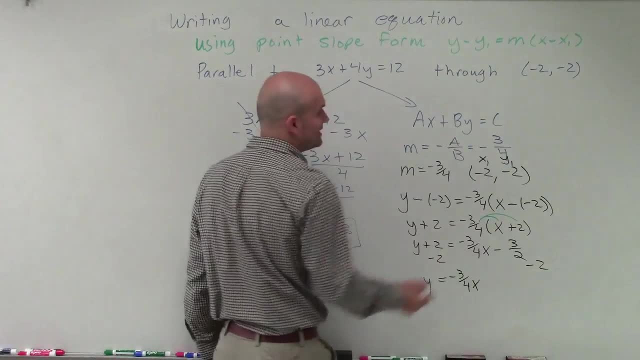 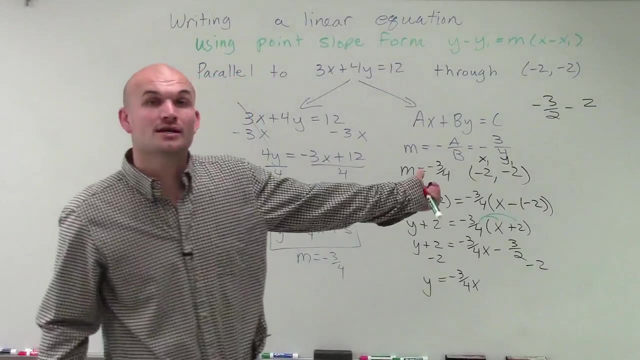 equals a negative 3 force X. and now I need to do negative 3 halves minus 2. well, when you're subtracting a fraction minus a whole number, we got to make sure we convert it to another fraction. then we got to make sure we have the. 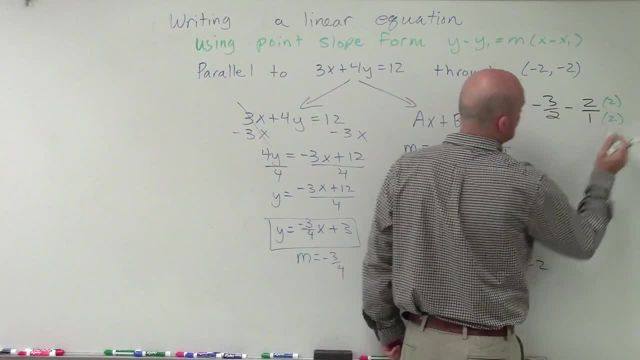 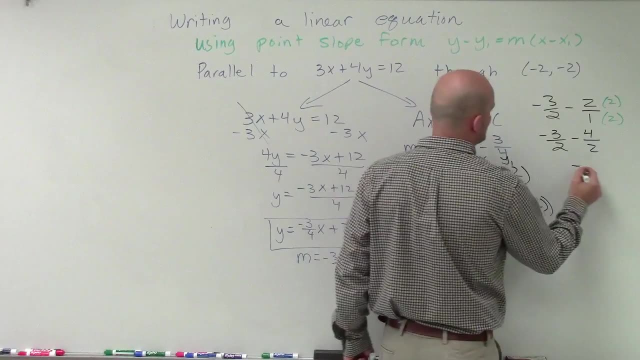 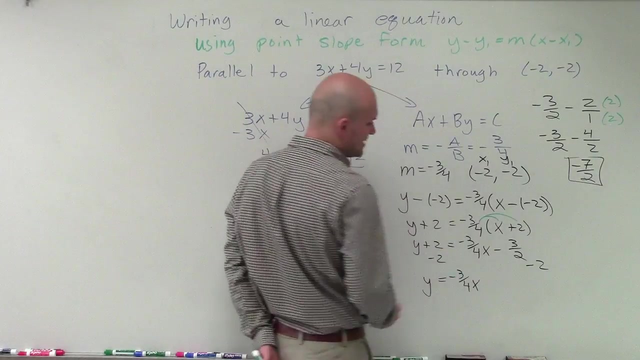 denominators be the same. so I'll multiply by 2 over 2. so therefore I have a negative 3 halves minus 4 halves. so therefore that equals a negative 7 halves. so therefore that's going to be our y-intercept, or a constant on our equation. so it's going. 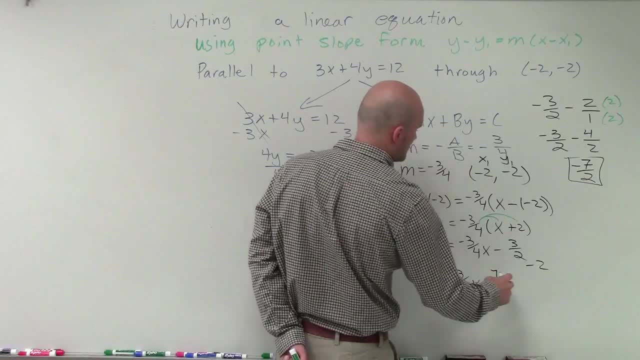 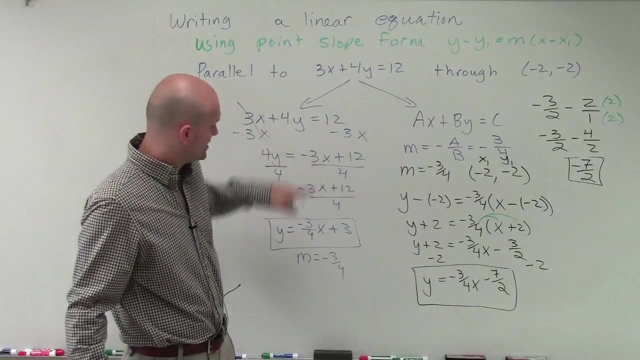 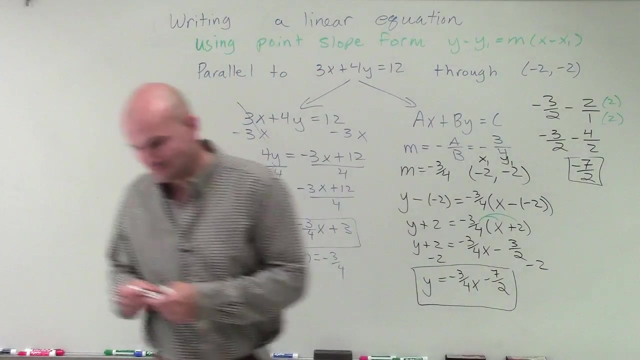 to be a negative 3 force X minus 7 halves. so there you go, ladies and gentlemen. that is the equation that is parallel to our equation in standard form, because I converted it and notice that they have the same slopes, but this equation goes to the point: negative 2, negative 2. thanks, you.